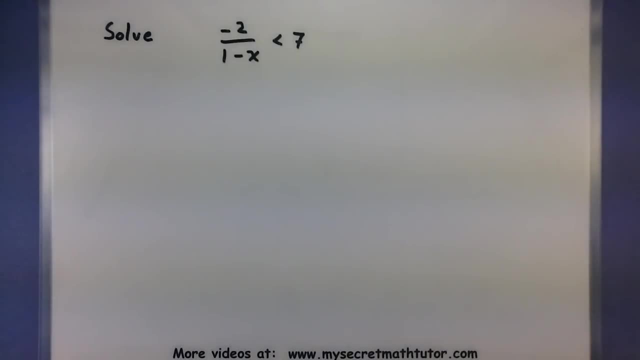 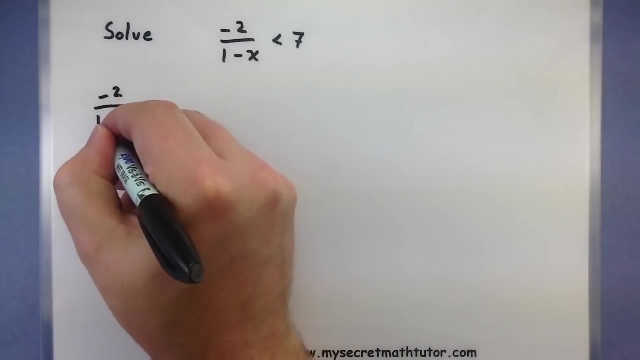 So in the first example I want to solve, a negative 2 divided by a 1 minus x is less than 7.. Okay, and I'll start right with step one and I'll try and get everything over onto one side. So let's go ahead and subtract a 7 from both sides, So negative 2: 1 minus x. 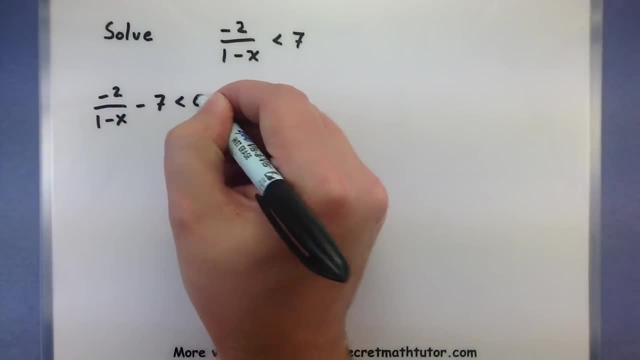 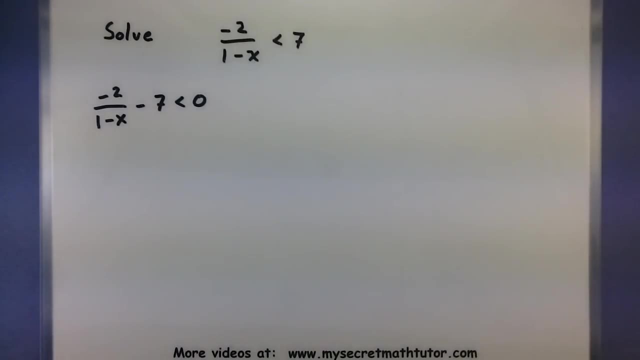 minus 7 is less than zero. Okay, that means that all I need to know now is whether this entire thing is either positive or negative, and you know, we'll find that out in just a bit. All right, so now that everything's over on one side, we need to combine it into a single fraction. Now that often involves 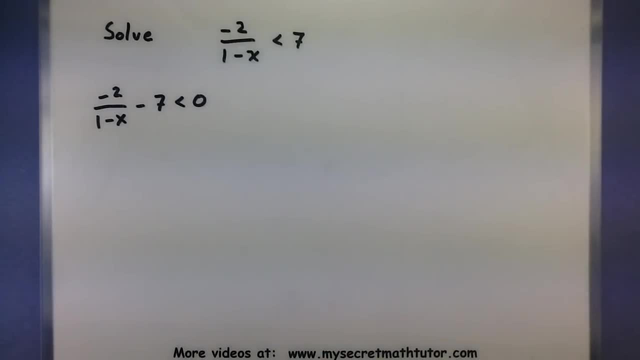 say finding a common denominator and putting them together. So we'll imagine this is 7 over 1 and we'll multiply the top and bottom by 1 minus x. All right, so this one doesn't change Minus. this one will be multiplied by 1 minus x and on the bottom, 1 minus x. 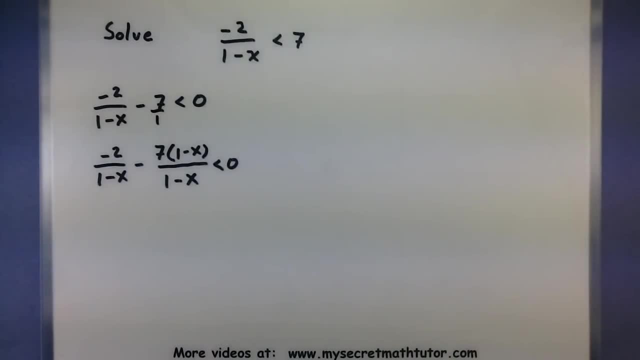 All right, looking better. Now that they have the same denominator, let's go ahead and put the tops together. So negative: 2 minus a. 7.. 1 minus x. all over, 1 minus x. All right, looking great. We need to do a little bit more simplifying. Let's go ahead. 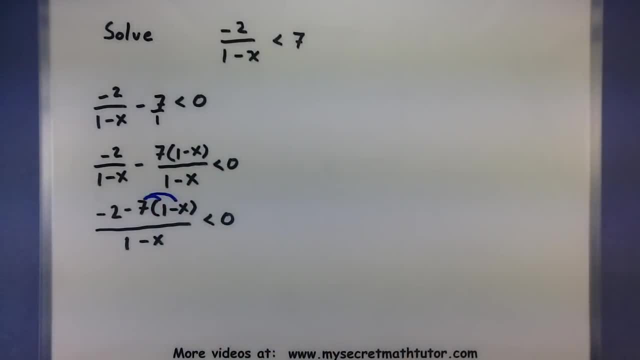 and distribute our negative 7 in, Let's see what we have. So negative 2 minus a 7 plus a 7x. Watch those signs. All right, almost done combining as much as we can. Now let's go ahead and continue. 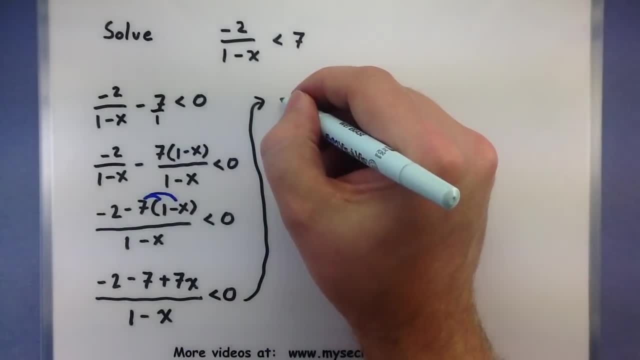 our work up here. So I have a negative 2 and a negative 7.. That would be a negative 9.. I have a positive 7x all over 1 minus x. So now that we have it into a single fraction, I need to start. 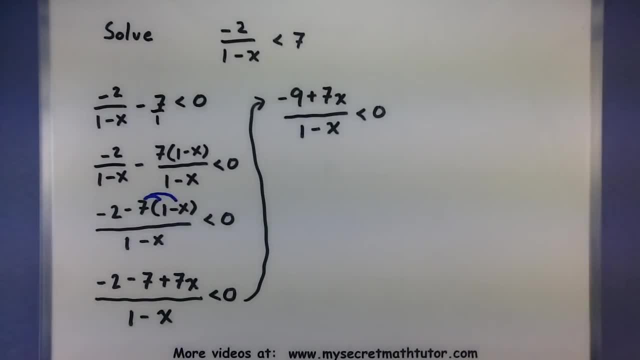 drawing out my critical values, We'll first figure out where the top is equal to 0 and where the bottom is equal to 0.. Okay, so let's do the top. Where is the top equal to 0?? We can literally just grab the top of our rational here and set it equal to 0 and solve directly. 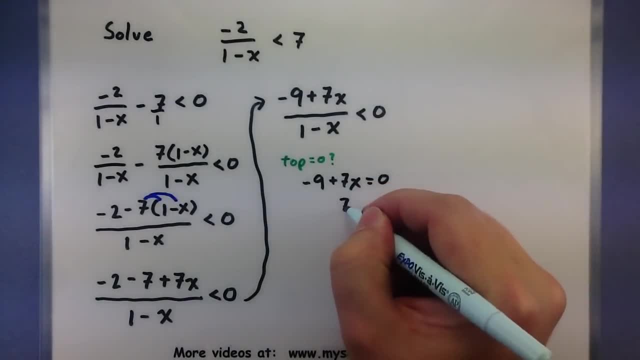 See solving this. I'd move the 9 to the other side and then divide everything by 7.. Oops should be a 7.. There we go. Okay, so we will take this as one of our critical values. Now let's find out where the bottom is equal to 0.. 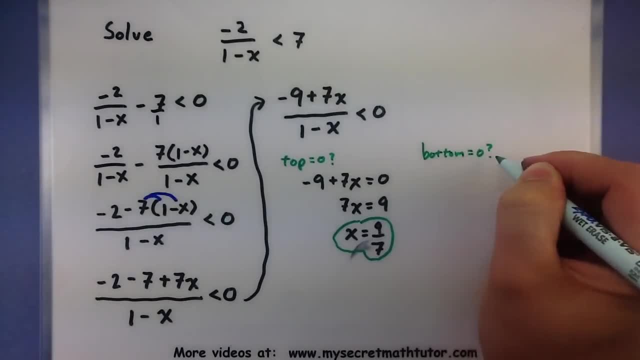 I'll go ahead and do that. And again, you can literally just grab the bottom part, set it equal to 0 and solve directly. Okay, so if I move the x to the other side, 1 is equal to x. So it's around these two values that I want to test things out, So things that. 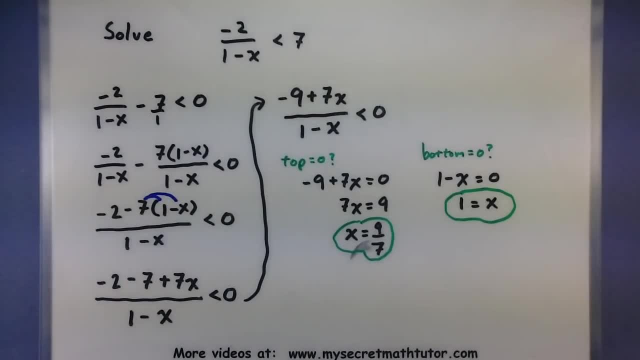 are, say, less than one, greater than one, less than 9 sevenths, greater than 9 sevenths. That's what I need to know about. So let's take these and figure out what our critical values are. Let's take these and put them into a table. 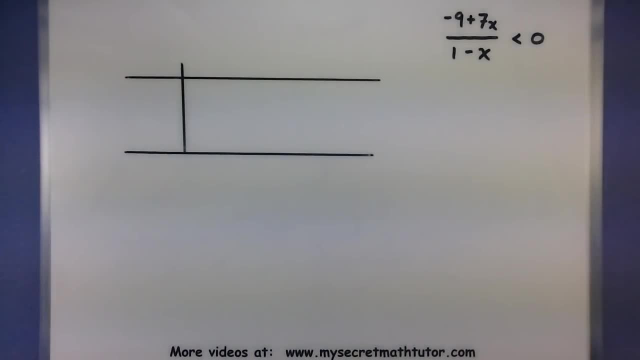 So I've already started to set up that table And here's some things that you want to make sure you do when setting this up. The top part of this table you want to treat like a number line. You want to put those critical values on that number line. 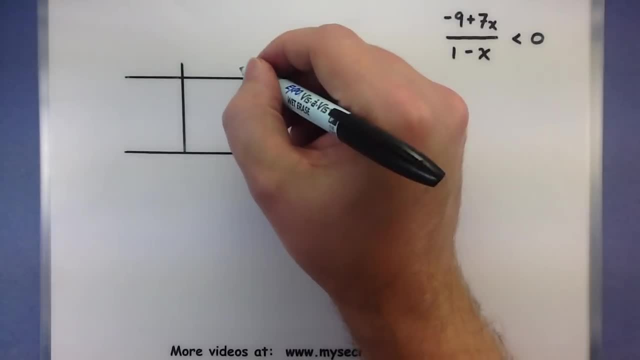 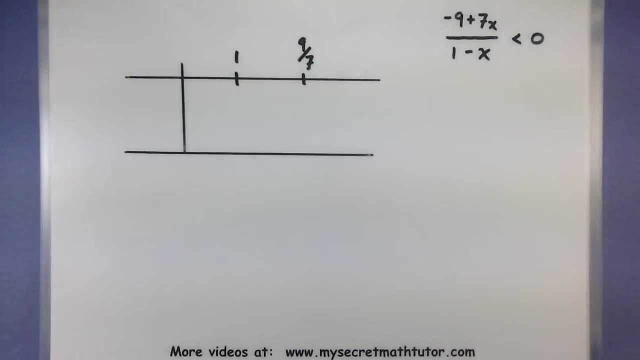 from smallest to largest. So of my values, the smaller one is at 1. And the larger one is at 9, 7ths, Okay, And what we'll be testing is values around each of these And we'll be testing them into, say, 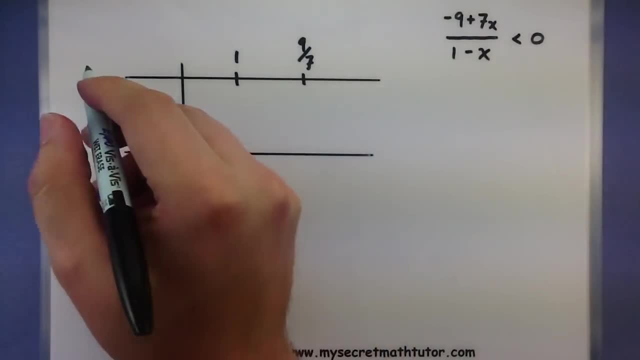 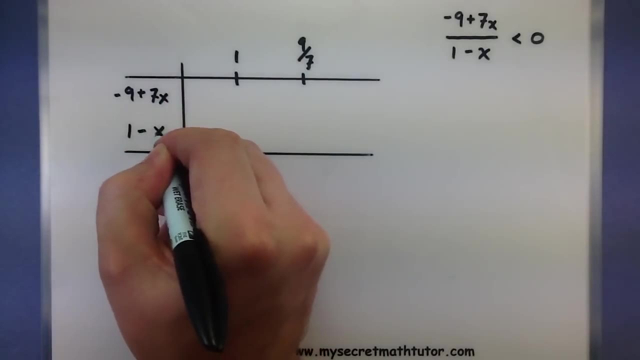 the top and bottom parts of our expression over here. So we'll be testing them into negative: 9 plus 7x. We'll be testing them to 1 minus x, And what we're really looking for is, you know, is the result positive or negative? 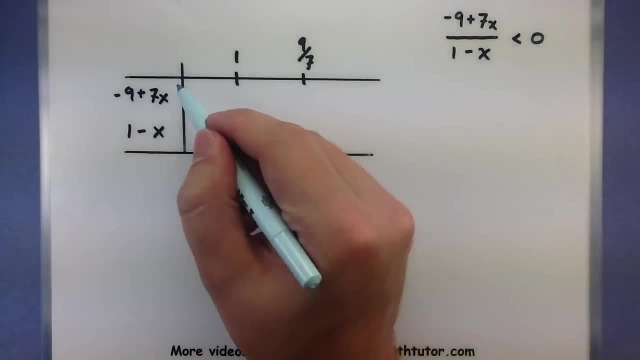 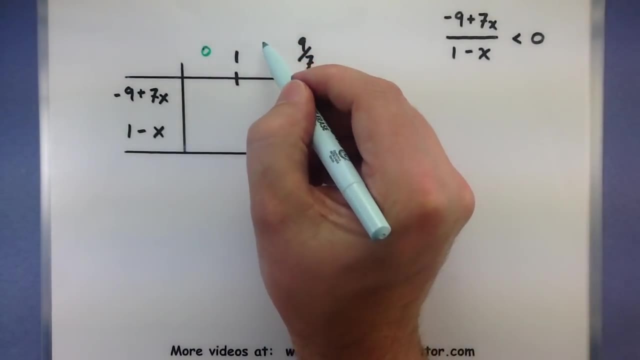 So let's just start off by picking values around each of these. So I need something that is less than 1.. Let's use a test value of like 0. Something between 1 and 9 7ths. Not a whole lot in there, but let's go ahead and grab 8 7ths. 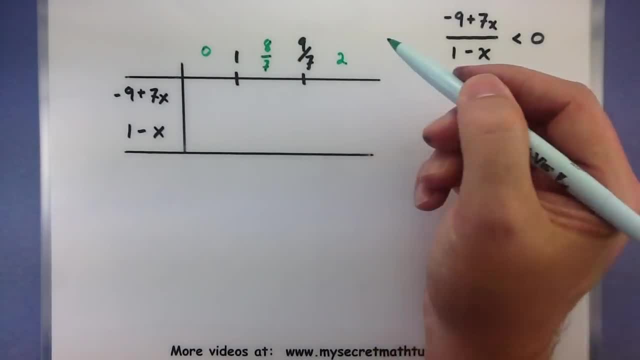 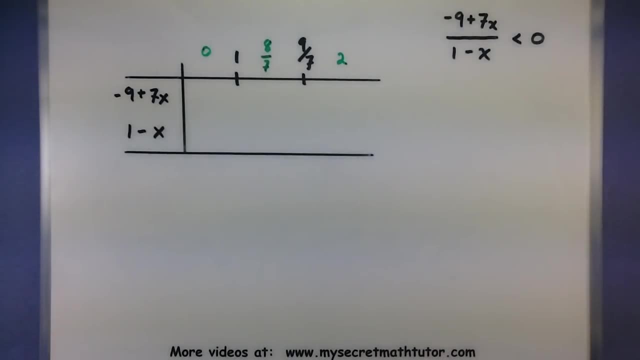 Something larger than 9 7ths 2.. So it's those green values that we'll be plugging into here. All right, let's see what we get. So if I was to take a 0 and plug it into my x for the top part, 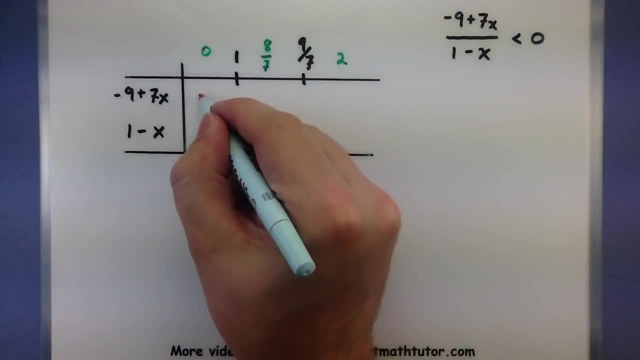 I'd have a negative 9 plus a 0, and the result is a negative value. Well, what would happen? What would happen if I took an 8- 7ths and I plugged it in there? Well, that'd be a negative 9 plus 8,. 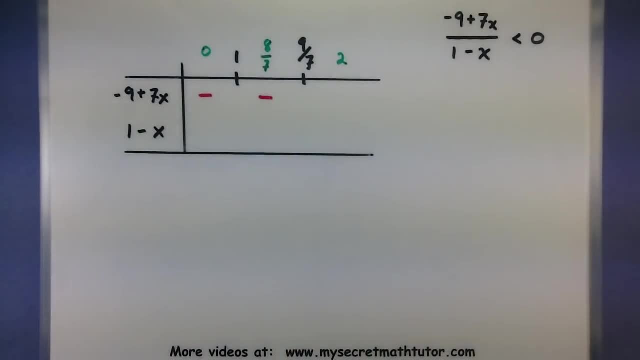 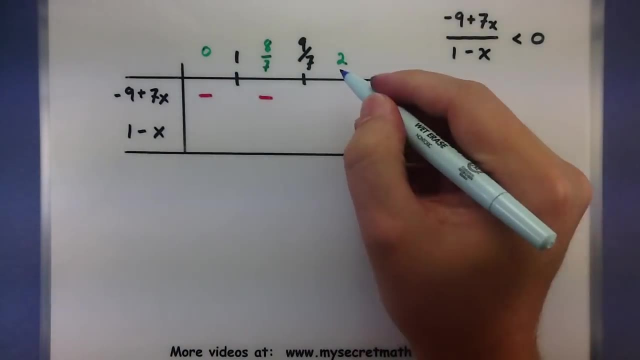 and the result is still negative. All right, and then one more. If I was to take 2 and plug it in here, that'd be a negative 9 plus 14, and that would be positive. Okay, so now I'm keeping track of the sign. 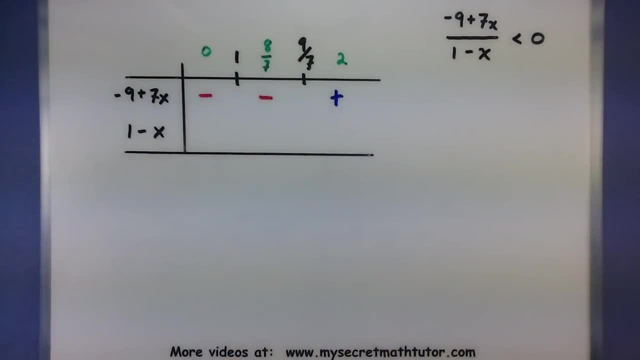 of what's happening to that top part. Now let's do the same for the bottom part. Okay, so putting in a 0 for x, I'd have 1 minus 0. That'd be positive 1 minus 8 7ths. 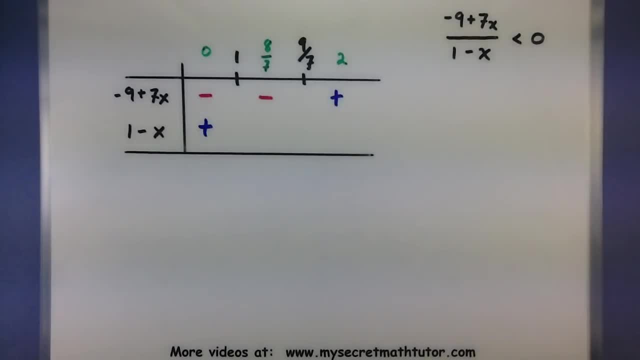 So 8 7ths is just a hair larger than 1.. So 1 minus something just a little bit bigger than 1 would be negative, And 2 minus 1 would be negative. Okay, now that I know the sign of each of the pieces. 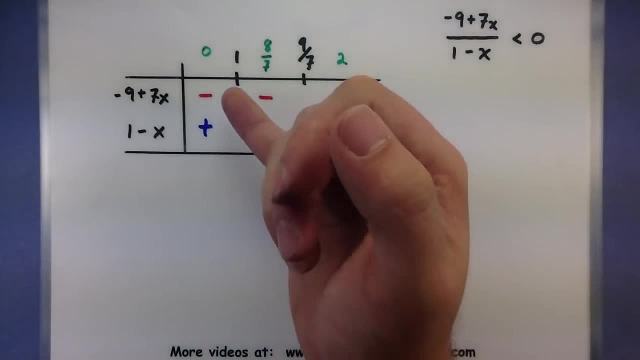 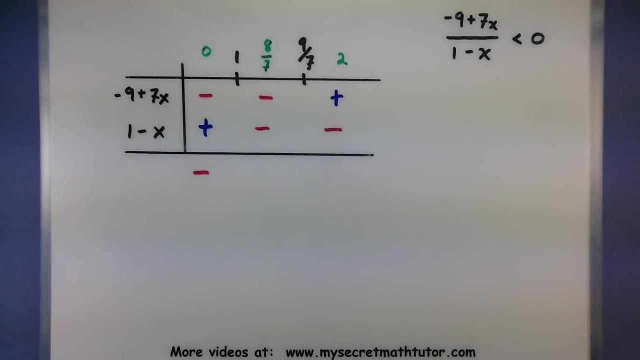 I can see that in my expression they're being divided. So think, in this first interval I'll have a negative divided by a positive. The result will be negative. In that middle interval I'll have a negative divided by a negative. 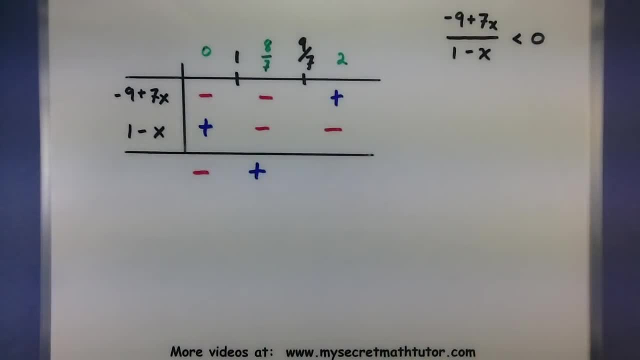 So the result there will be positive, And on the last interval, a positive divided by a negative, The result is negative. So now I know exactly what the rational expression is doing on every single one of my intervals. So which ones do we want? 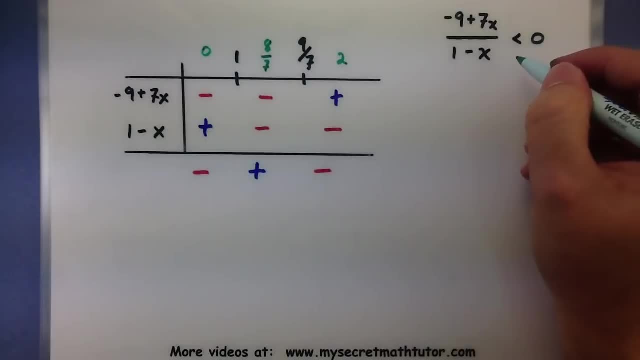 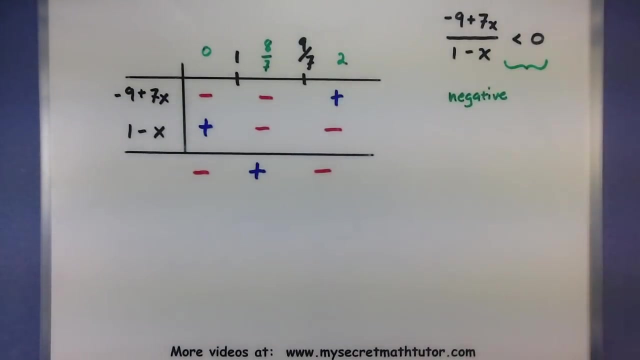 Well, it all depends on the direction of our inequality. Notice how, up here, when we put things together and got everything to one side, we have less than zero. Less than zero is our indication that we want negative values. So let's go ahead and write down the intervals. 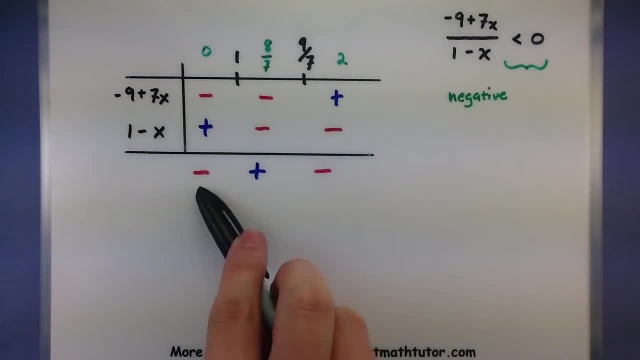 that involve those negative values. So we got two of them. Looks like one here and one here. This first interval involves all the numbers, say, from negative infinity all the way up to 1.. And this other interval that gives us a negative is from 9- sevenths. 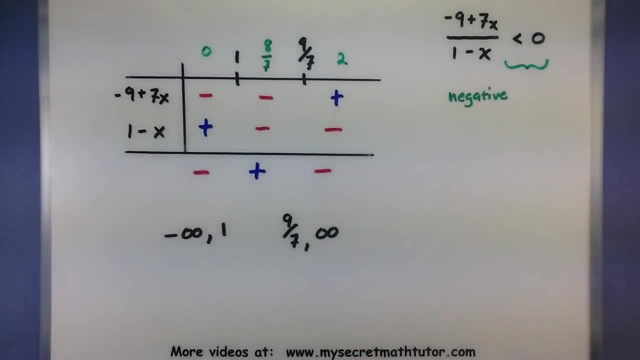 all the way up to infinity. Now we're on to the very last step. I need to check all of my endpoints to see which ones I should include, which ones I should not include, Any time we're dealing with, say, infinity or negative infinity. 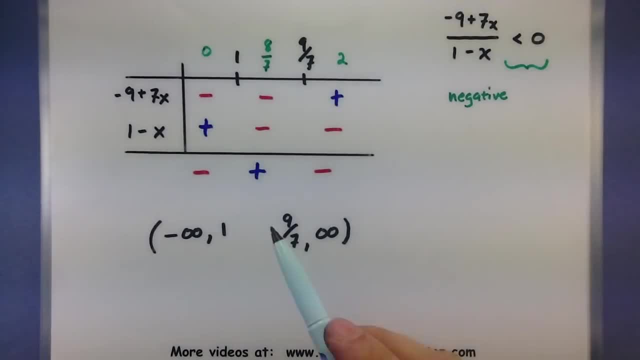 those will never be included, so we'll use a parentheses to show that. Should I include the one? Well, no, because it makes the bottom zero. We'll never include any values that make the bottom zero. And how about 9 sevenths? 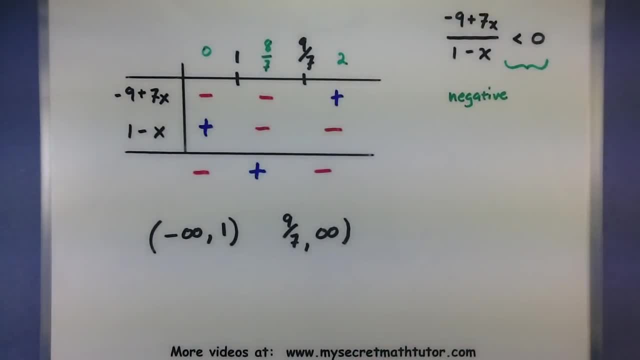 If I was to use that in the original, I would get a zero in the top, and this would actually just be zero less than zero. In this case, we're dealing with a strict inequality, so I don't even want to include places where it's equal to zero. 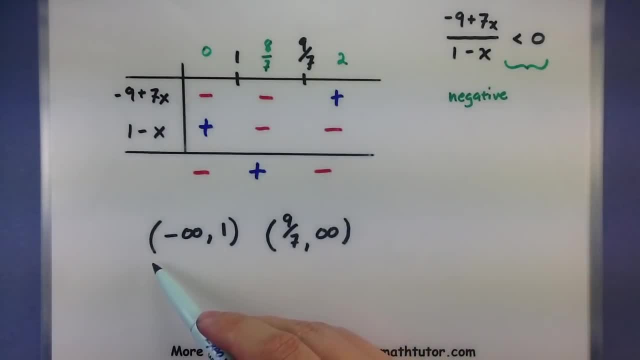 So we won't include that one either. So my solution interval is everything from negative infinity up to 1, or from 9 sevenths up to infinity, And then this one's done. So you can see there is a lot of work in here. 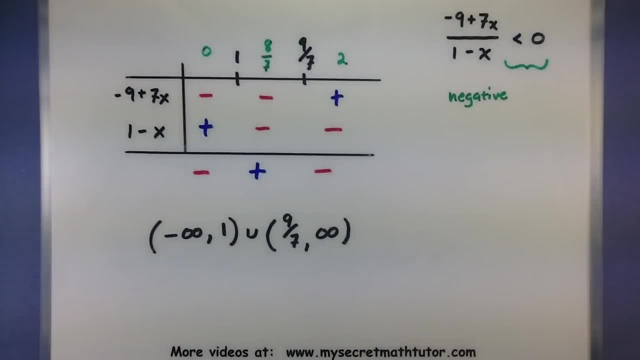 but it's manageable with the table, as long as you're keeping track of all the signs. Let's do one more example, just to make sure you have this process down, And this one will be a little bit bigger. Alright, We want to solve 5 divided by. 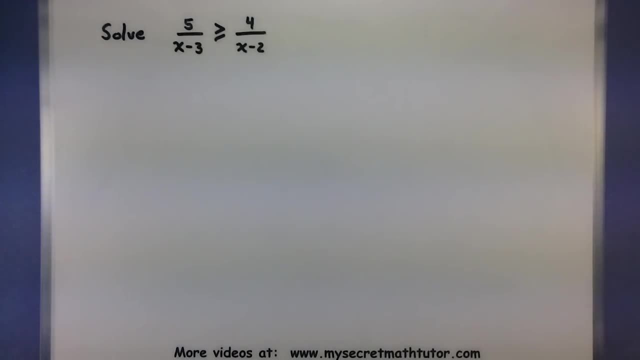 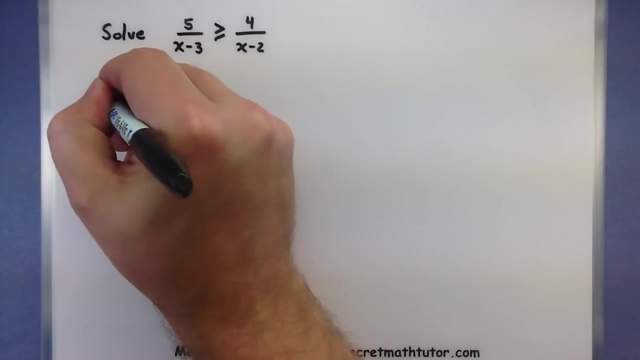 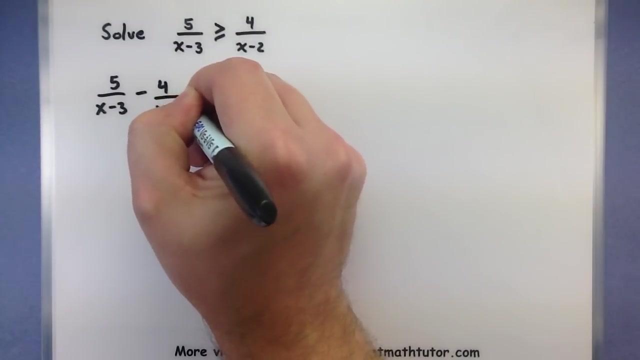 is greater than or equal to 4 over. Alright, Let's start off just like we did before. Let's get everything onto one side. So I have 5 x minus 3 minus x minus 2.. So we want to know greater than or equal to 0. now 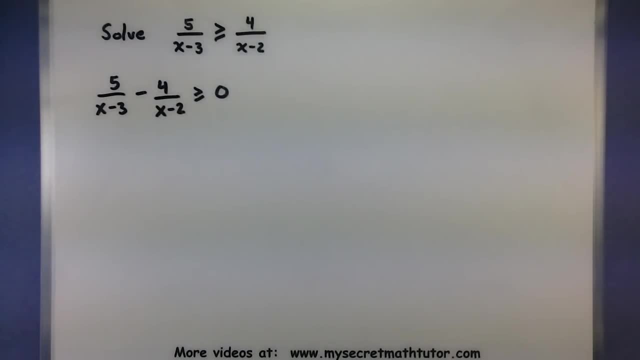 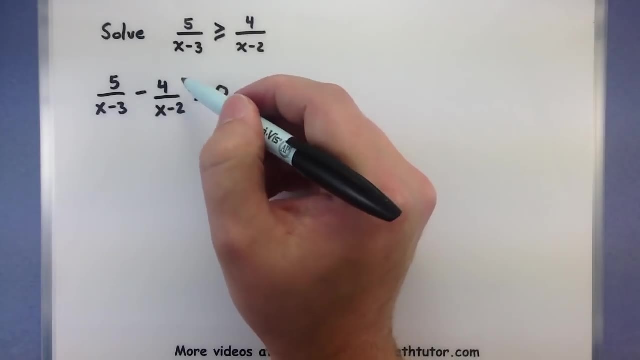 Alright, Like before, we're going to put these together, but we need a common denominator first. I'll multiply this rational on the top and bottom by an x minus 2 and this one on the top and bottom by an x minus 3.. 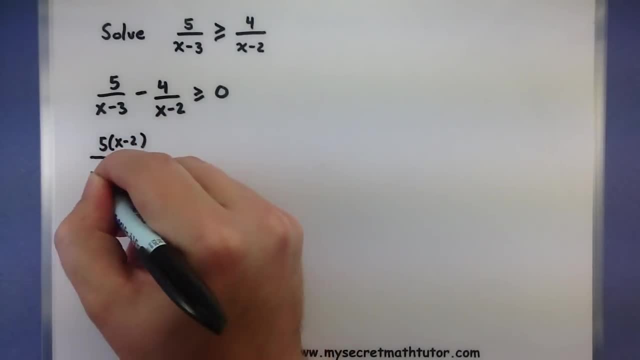 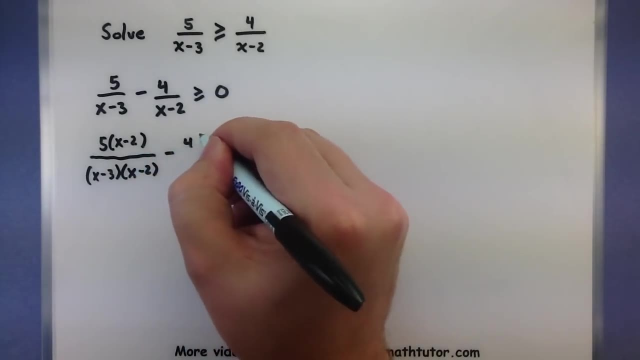 So 5 x minus 2 all over. So now I have an x minus 3 and an x minus 2 on the bottom minus, and then we'll do the other one, x minus 3.. So that's going on the top and on the bottom. 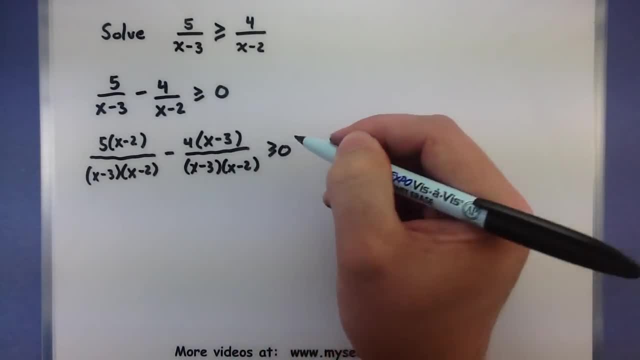 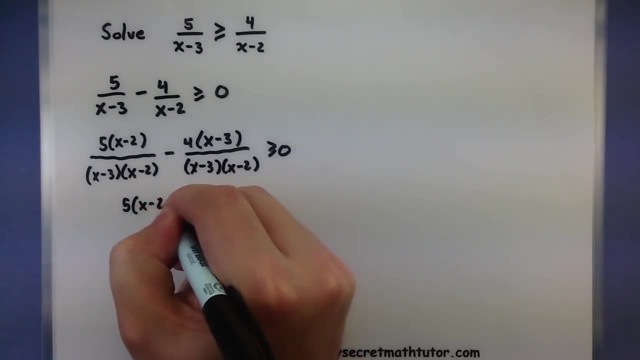 And now we can see that both of our denominators are exactly the same. So things are looking good. Now let's go ahead and just put the tops together: So 5 x minus 2 minus 4 x minus 3, and all of this is over the same. 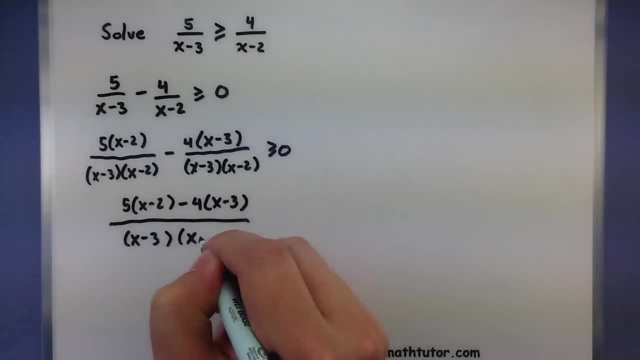 denominator x minus 3 minus 2.. Okay, Looking pretty good, We are still greater than or equal to 0.. We just need to simplify the top of this just a little bit more so we can continue on. So we're going to distribute in our 5. 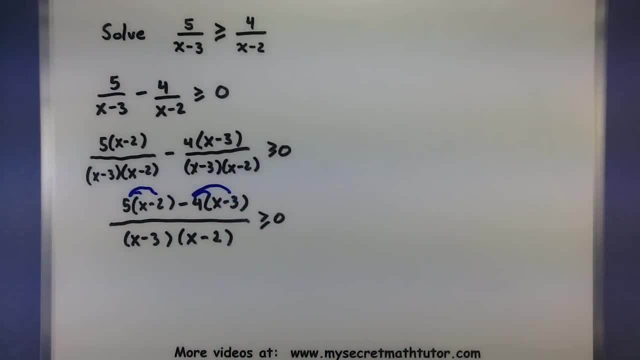 and we'll distribute in this negative 4.. 5 x minus 10 minus 4 x plus 12, all over x minus 3 x minus 2 greater than or equal to 0.. Okay, A lot of stuff lying around in here. Let's go ahead and continue. 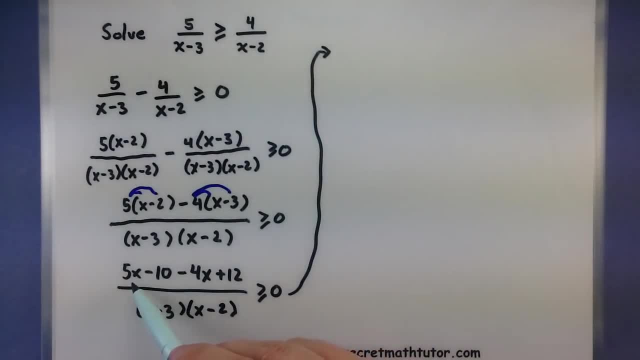 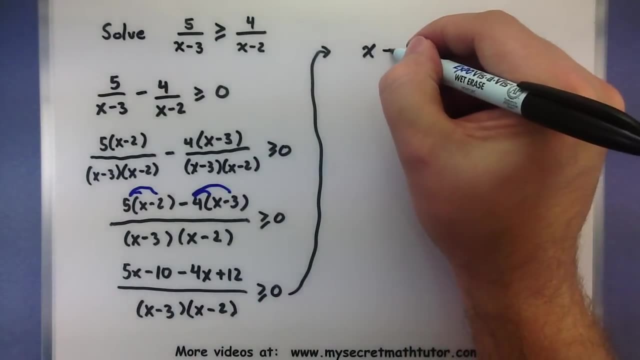 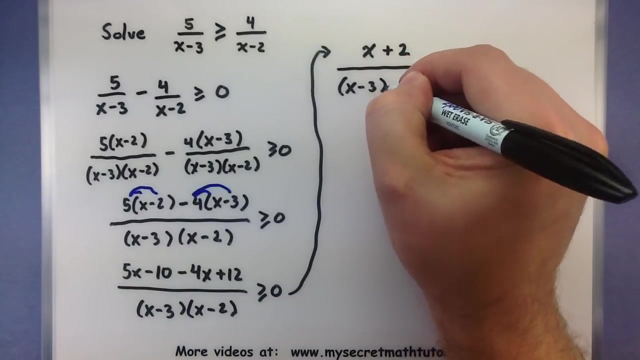 the rest of our work way up here. So combining a 5 x and a minus 4 x would give me a single x Negative. 10 plus 12 would be a positive 2. So that would completely simplify the top And the bottom. well, we're. 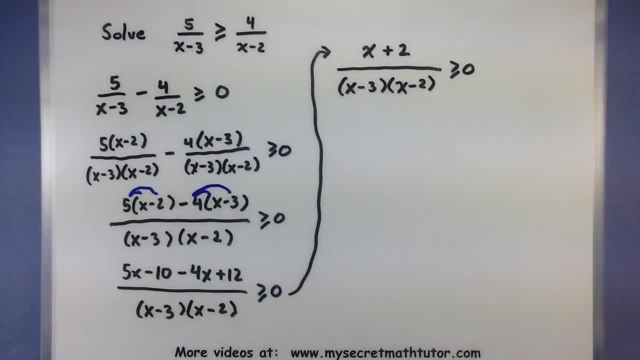 just going to leave that factored. okay, It'll actually make finding the critical values from the bottom a little bit easier. Okay, So we've shifted everything over to one side, made it into a single fraction. Now let's find out where the top. 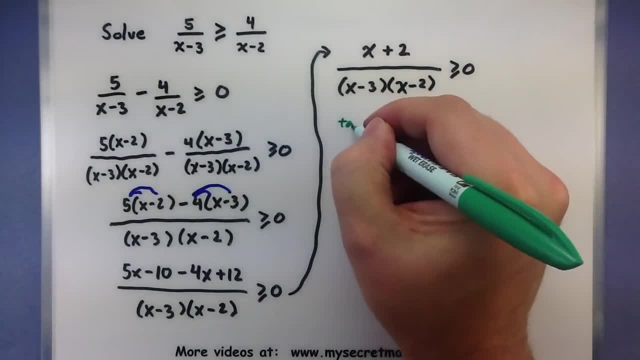 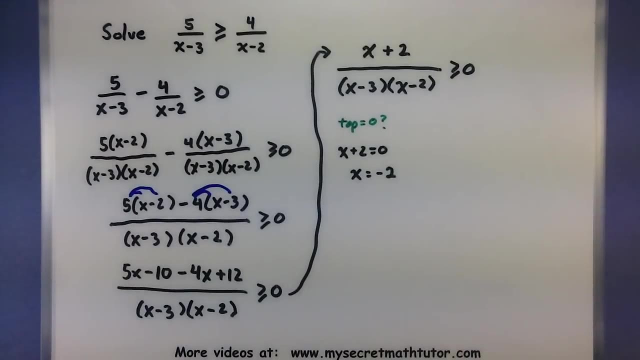 and the bottom are equal to 0.. Alright, So let's go ahead and grab the top part of this, Set it equal to 0.. Solve directly And it looks like one of our values is at a negative 2.. So we'll hold onto that. 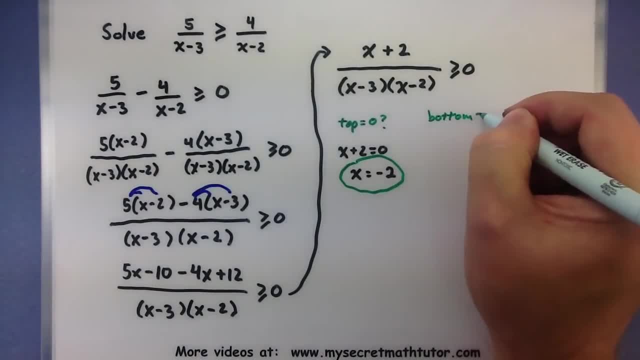 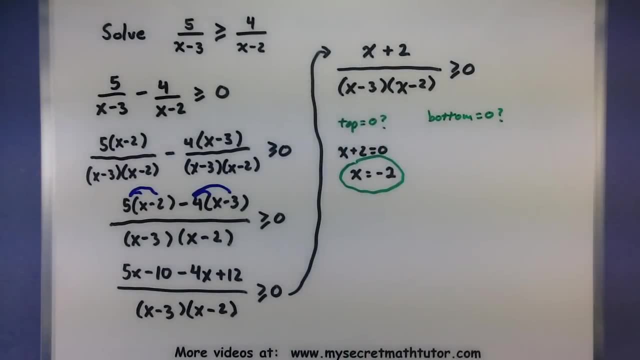 Now, where is the bottom equal to 0? Well, I actually have two factors in the bottom that I need to consider, So we can take each of those. So, x minus 3, where is it equal to 0?? Well, when x equals 3.. 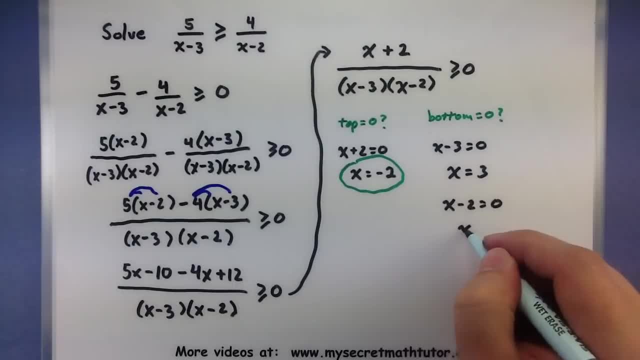 And how about x minus 2, where is that equal to 0?? Well, when x equals 2.. So this one. I end up with a few critical values And we'll need to check around every single one of those. okay, But make sure you got them all. So you got one of them. 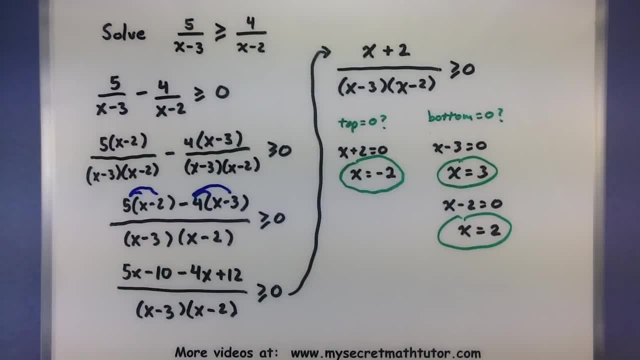 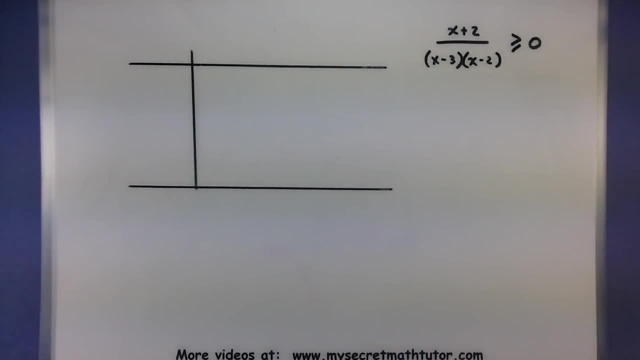 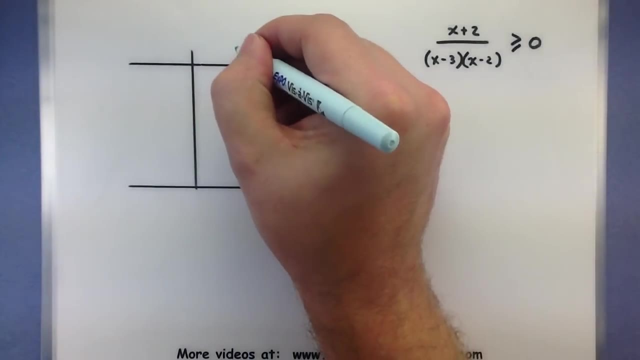 from the top and a couple from the bottom. Alright, Let's take these values and put them into our table. Remember that as you're putting these values into the table, write them from the smallest value you found to the largest. So our values are at. 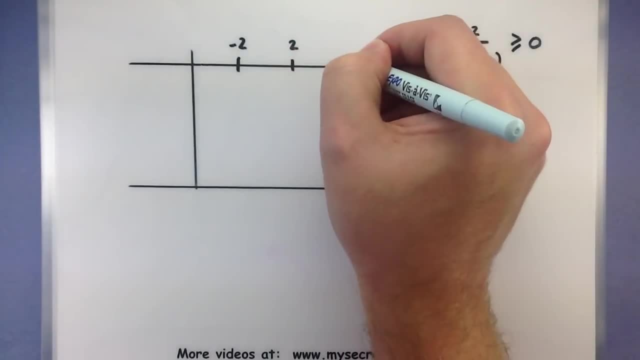 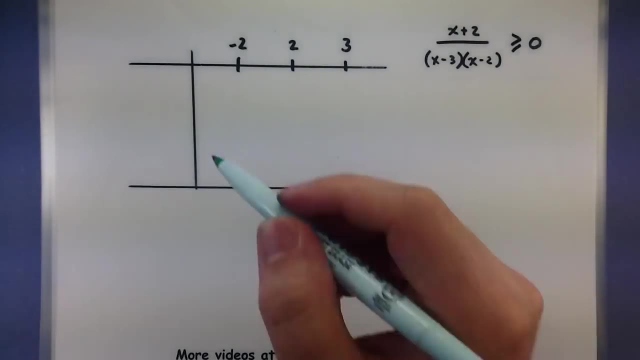 negative 2,, 2, and 3.. And if you want, you can go ahead and write down the values. we'll be testing around these. So something less than a negative 2, you could imagine maybe a negative 3.. Something between 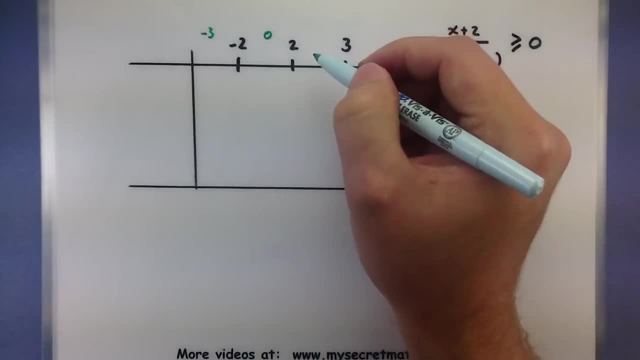 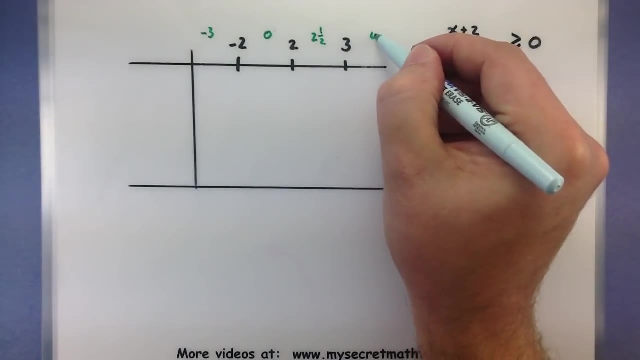 a negative 2 and 2, 0 works pretty good. Something between 2 and 3,, maybe 2 and a half, Something larger than 3,, maybe a 4.. Alright, so each of these needs to be tested into all of the. 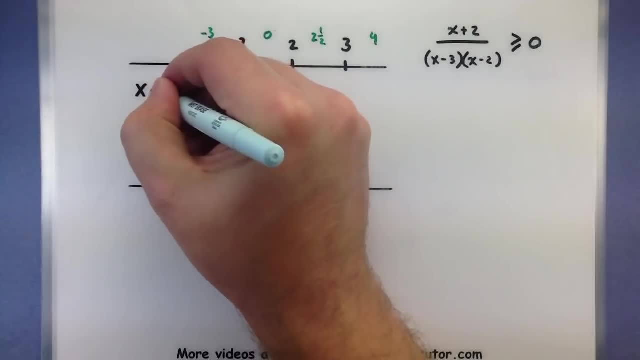 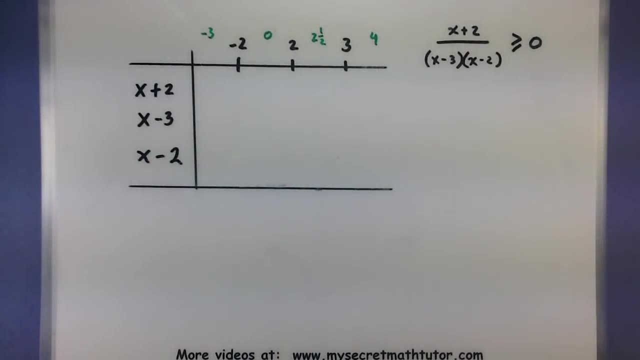 parts of our rational. So we'll test things into our x plus 2 part, our x minus 3 part and our x minus 2 part. Alright, Now, one by one, let's go ahead and start plugging these in. 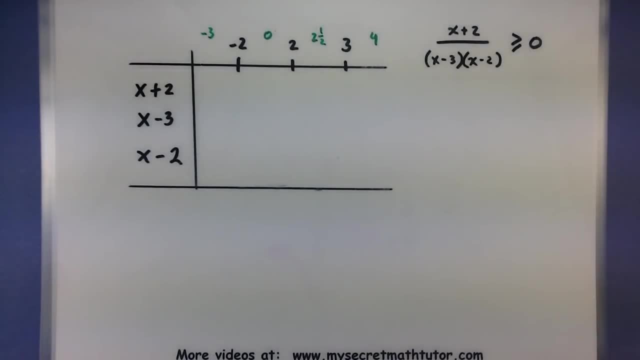 So what happens if I take a negative 2 and I put it, I mean a negative 3, and I put it into x plus 2? Well, negative 3 plus 2 would give me a negative value. Alright, moving on. 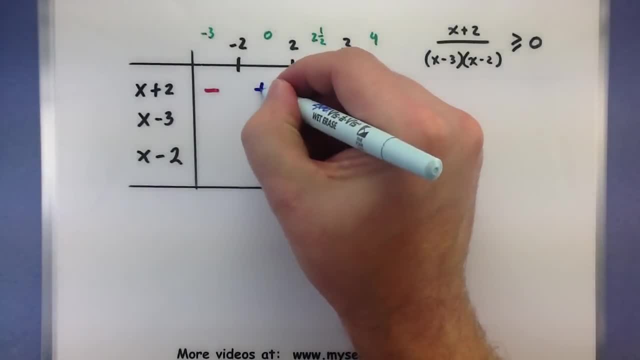 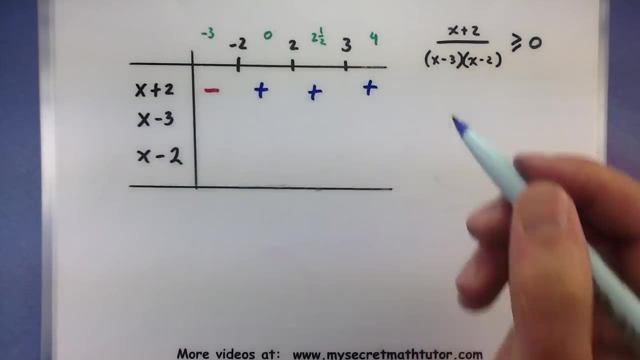 If I put a 0 in there, 0 plus 2 would be positive. Keep going. 2 and a half plus 2, still positive. 4 plus 2, still positive, Positive 6.. Okay, so that part is done. 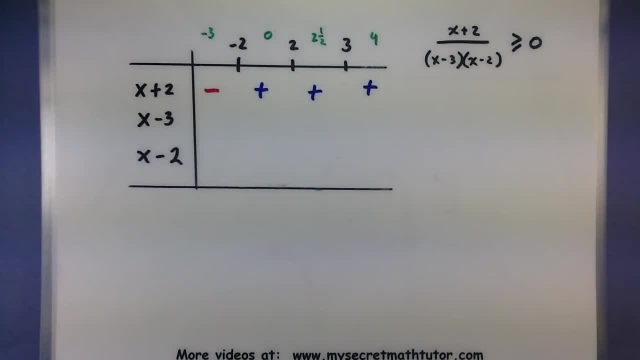 Now let's go ahead and test out a negative 3 into here. So negative 3 minus 3, negative 0 minus 3 would be negative 3.. 2 and a half minus 3, that's close, but it's still negative. 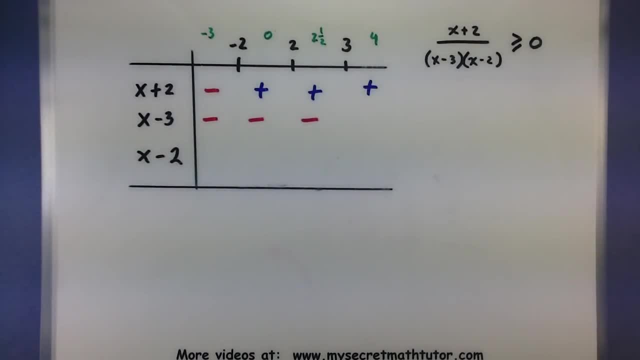 And last, a 4 minus a 3 would be a positive 1.. So positive, Okay. one last piece of the check, Let's see what it's doing. So negative: 3 minus 2 would be a negative 5.. 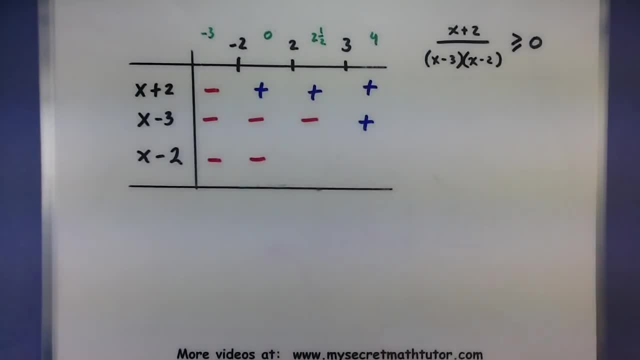 0 minus 2 would be a negative 2.. 2 and a half minus 2 would give us a positive 1 half. So make sure that part is positive. And last, 4 minus 2 positive 2.. So now that we know what each 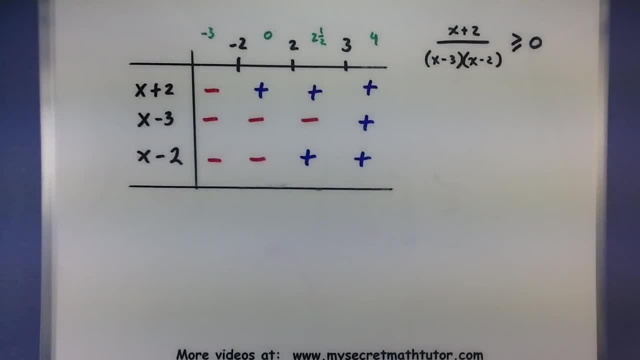 individual piece is doing on each interval. now we need to imagine putting all of these pieces together for our entire rational here. So as we're putting these together, we're going to do this column by column. So in this first interval I'm imagining a negative. 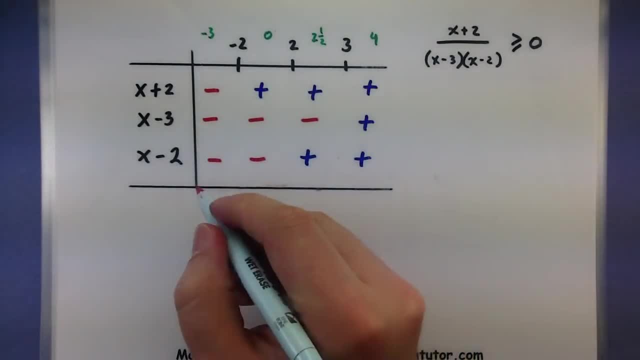 value being divided by a negative times a negative. So something like this: A negative being divided by a negative times a negative. Now, if you notice on the bottom, when you multiply two negatives together, they actually become positive. So what's? 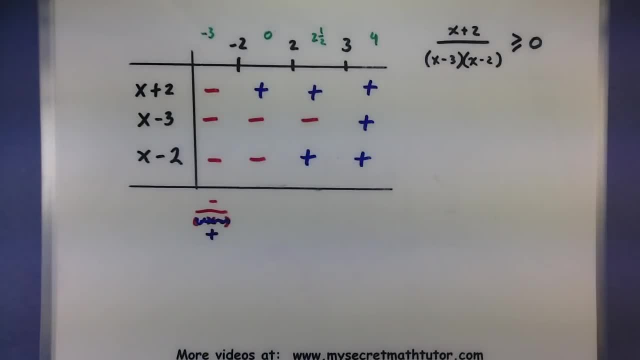 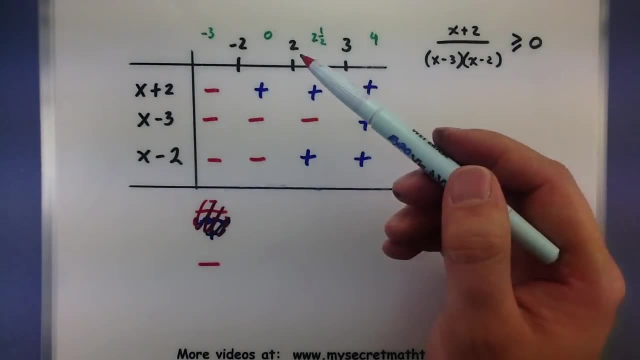 happening there on the first interval is I have a negative divided by a positive. The result is negative. Let's scratch out our work so we don't confuse it with the rest. On this next one, I'll have a positive divided by a negative times. 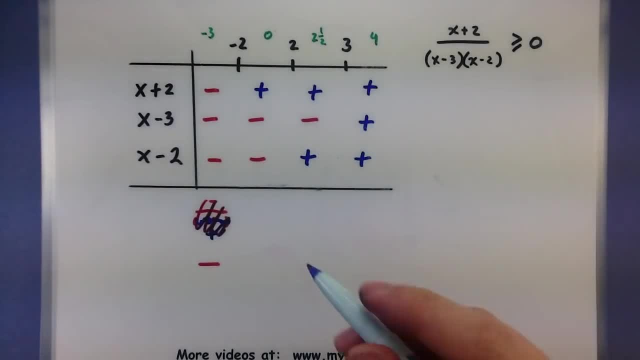 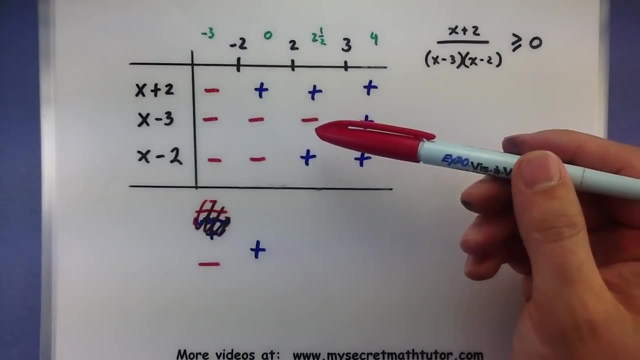 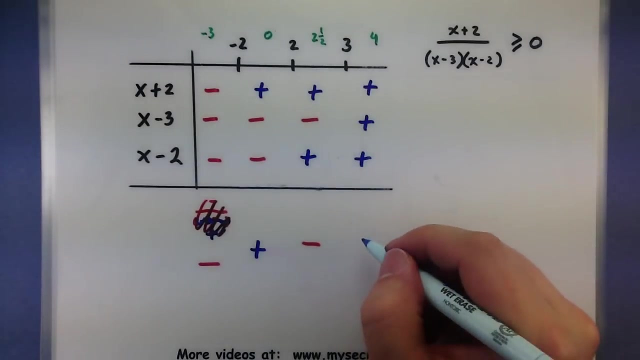 a negative. So that will reduce to a positive divided by a positive, That interval positive, Moving on Positive, divided by a negative times a positive Negative And for our last one, everything's positive. so combining it it better be positive. 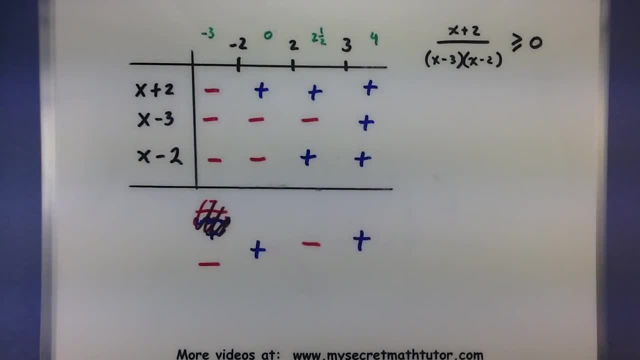 Alright, it's looking pretty good so far, Almost there. Now we need to figure out should we take the positive intervals or the negative intervals. Well, in this one, after we combine things, we have greater than or equal to zero. That's our clue that we want our 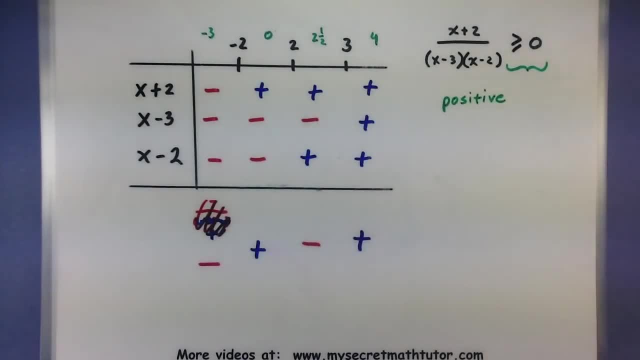 positive intervals, Things greater than zero. Let's say I have this interval between negative two and two. I have this interval from three all the way up to infinity. So let's first begin by just writing those intervals down. So from negative two up to two.